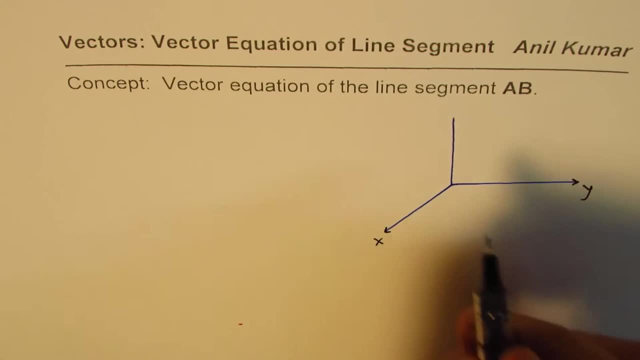 and we'll consider a line in this plane. So let us say that the line is kind of like this. Now, on this line, let us consider two points. Let's say point A is here and then we have a point B here. Let us say we are given these two points and we need to find vector equation of the line segment. 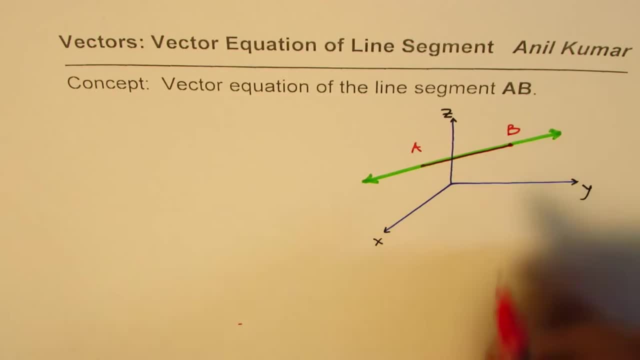 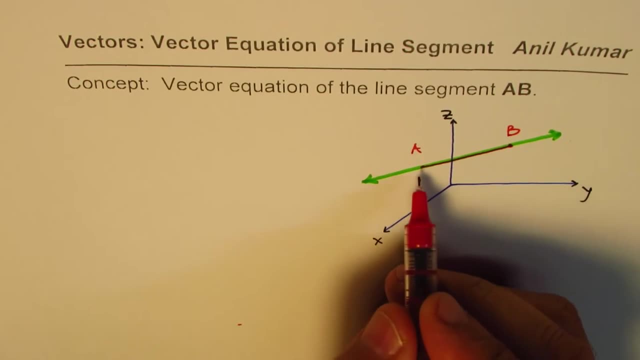 AB, that is this segment. So that is the exercise in which we are interested. Now what we can do is this: A, we know the position, vector A. so from the origin, let us say we have a vector R0 whose head is at the origin O and the tail is on the line. So tip of this vector is on the line. 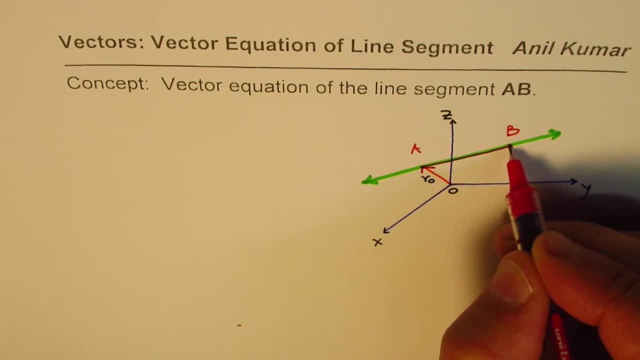 Similarly, point B has the position vector OB right. So this position vector OB, let me represent this by R1.. So R1 and R are the position vector. So R1 and R are the position vector. So R1 and R are the position vector. 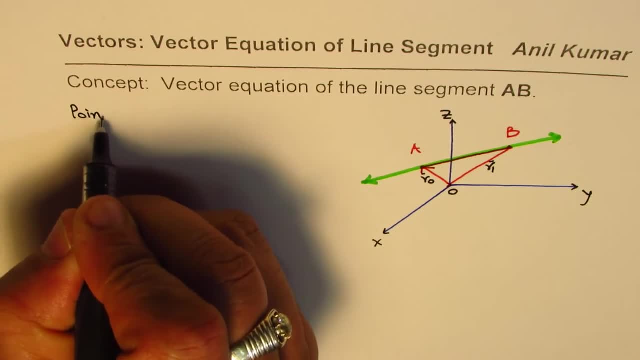 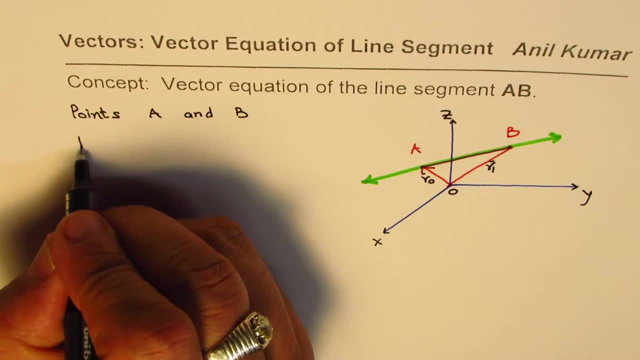 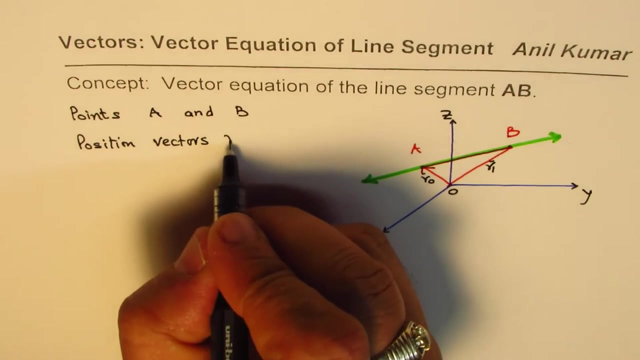 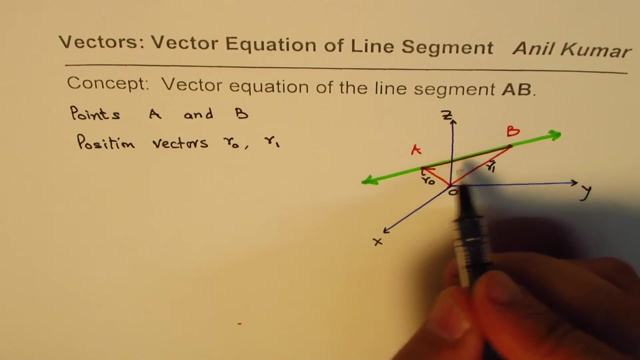 So we have points A and B, and then we have position vectors R0 and R1.. Now, with these position vectors, we can actually find the direction of this line. Let us say the line is L1, right, so what we are going to do? it's going to create another line here and let us say its this position vector here and Jing for these two lines, we can actually find the direction of this line. Let us say the line is L1, right, so what we are going to. do is, basicly, we are going toulo these two vectors, R1 and R1, and then here we want to use these two vectors for R1. So R1. we are going to implement those three coordinates into the player. we are going to set up a gleichly regular vector A into index, So that is a higher orschy or vídeos and case where R1 is care decisively. 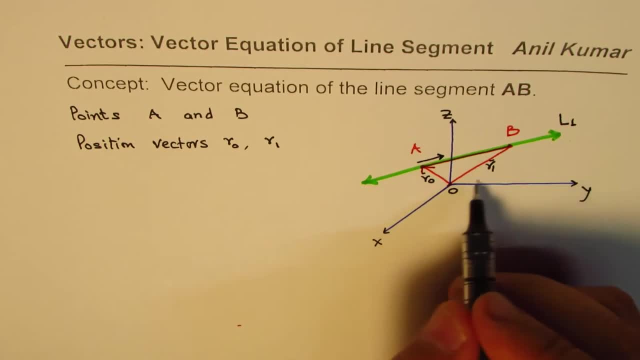 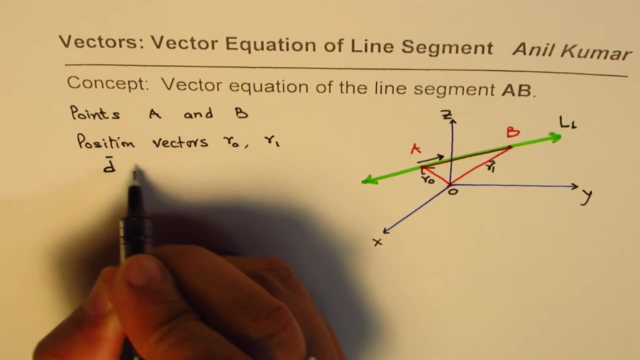 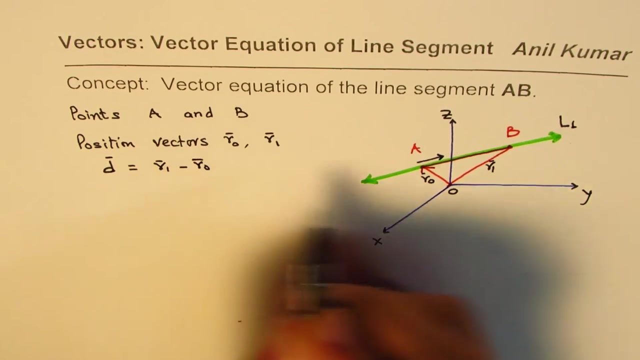 is the direction of this line. what is this direction? to find the direction. we can always find the direction. let's say direction vector d will be equals to r1 minus r0, right? so that gives you the direction from a to b, right? so that's the direction. 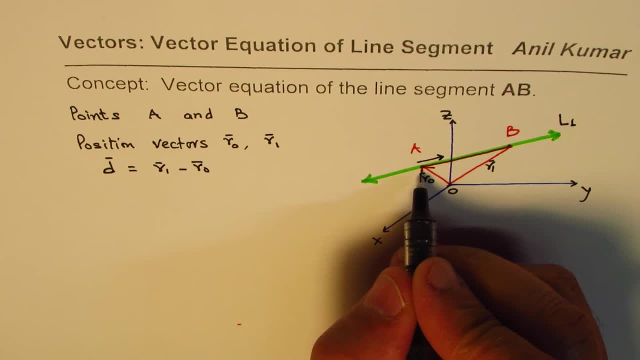 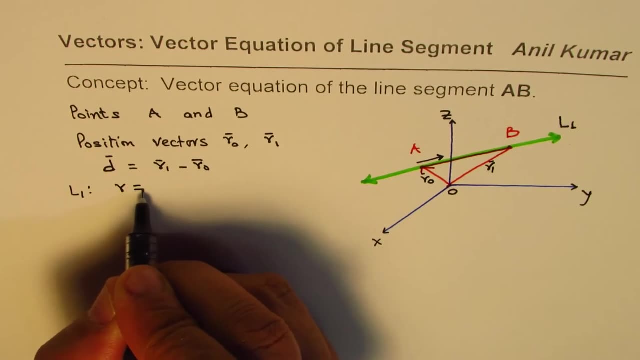 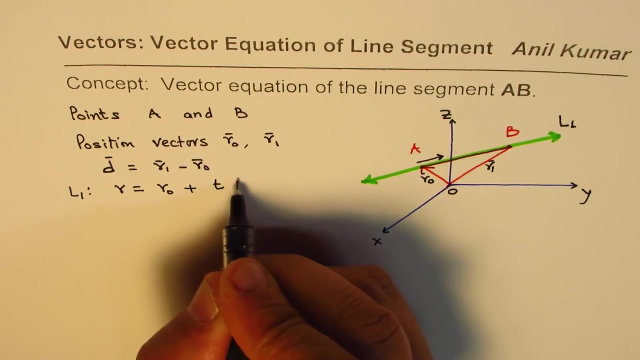 now, if i know the position vector a, then the equation of the line l1 can be written as: r equals to r0 plus any parameter. t times the direction, which is r1 minus r0, right r1 minus r0. so that is how you get. 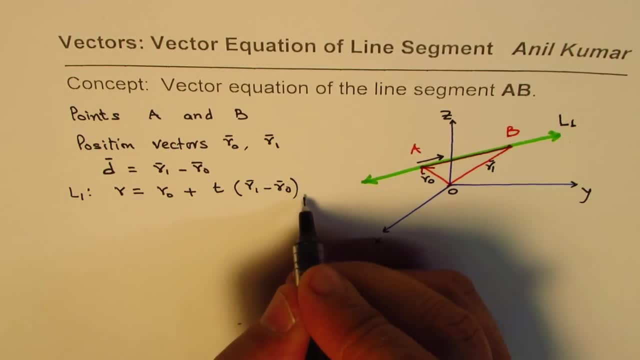 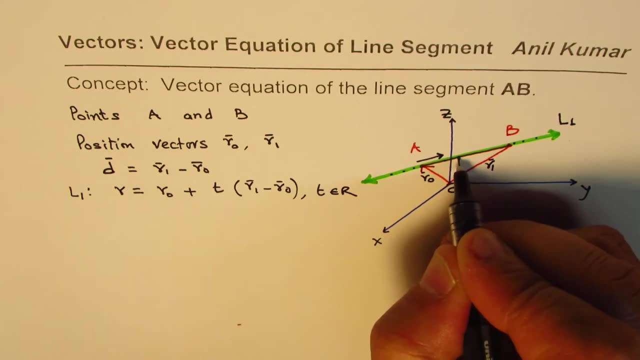 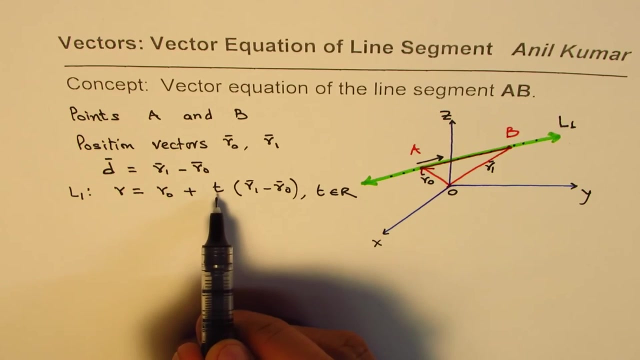 the equation of the line. so this represents the line. if t belongs to real numbers, then every point on this line can be associated with this equation, right? if t is positive, it is on the right side of a. if t is negative, these points will be on the left side of a, but that becomes the equation of the whole line. 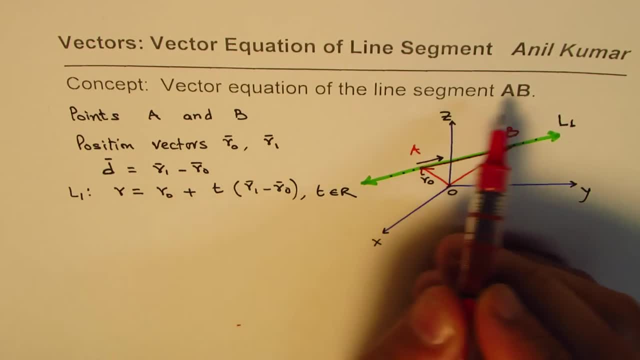 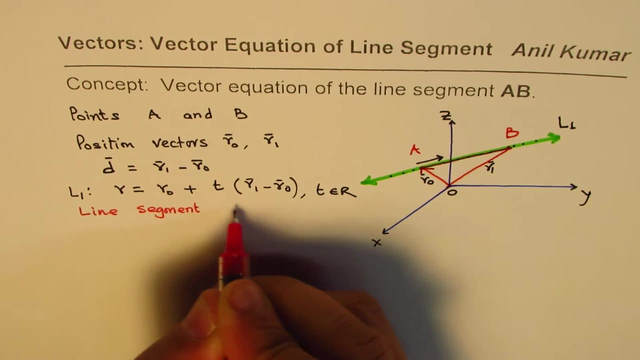 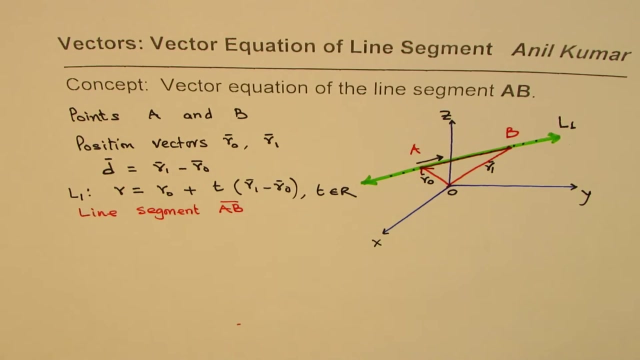 the question is: what is the equation of line segment a- b? so we are interested in line segment a b, right, so this segment we are interested in. what is the equation of this line segment? so what will observe here is: we can, of course, rearrange this, let's do that also, but before that, what we will do is that we'll see what really the line segment is. 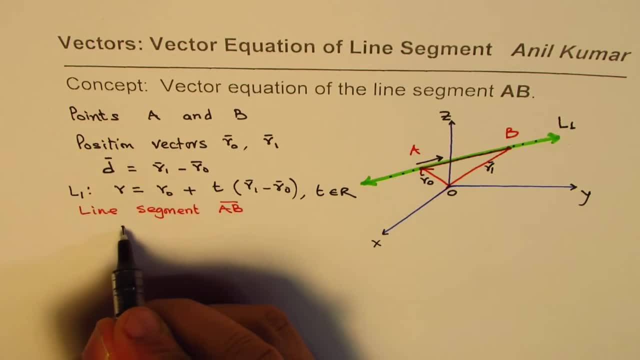 different from being this segment right, and this is segment b 했. this segment ab, we are interested to apply with a line of these corresponding Guilds, but know, line segment? we will see the equations here and now. this segment is not a line segment, so it's significant on the algorithm video in the opposite with an exemption line. that section, on the other hand, will call: reflection is the delt and not a line segment, line segment, just that equation. over here, when i will describe thector, however, i come across with a line segment which прекрас and pigs. the details now say universe, over here, where are the lines? evenly, and this is a line segment. 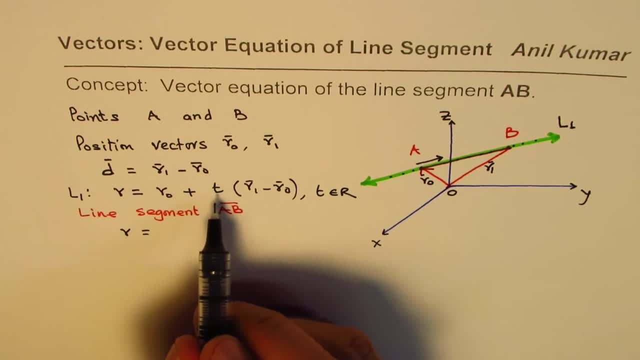 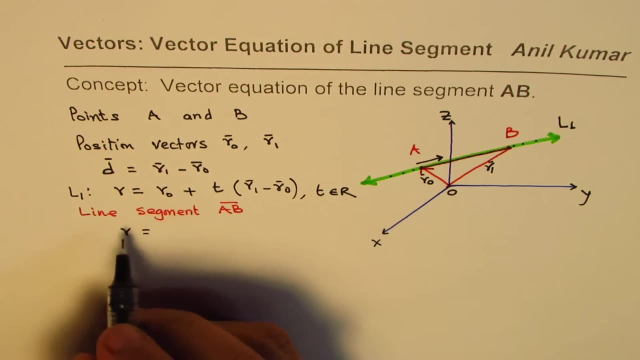 segment a, b is: if i take value of t as 1, where do i land? if i take t as 1, then if t, let us say if t equals to 0, then what do we get? if t is 0, we get r as equal to. 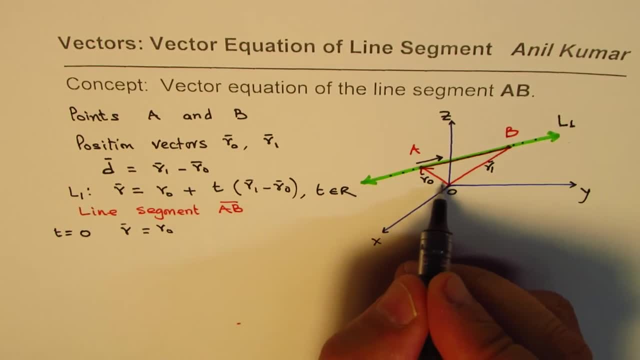 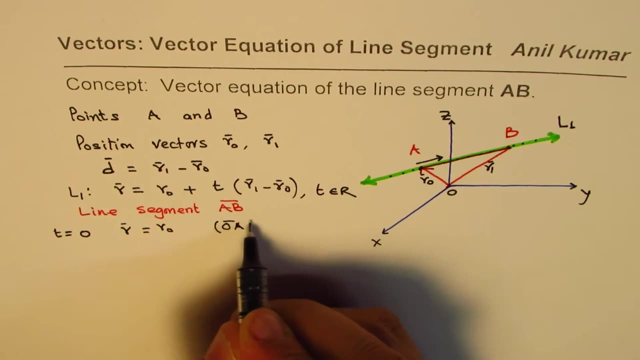 r 0 right. so that is a right. so that is the position which we get. o a. do you see that if t equals to 1, then r will be equals to r 0 plus t is 1. so we get r 1 minus r 0, right. 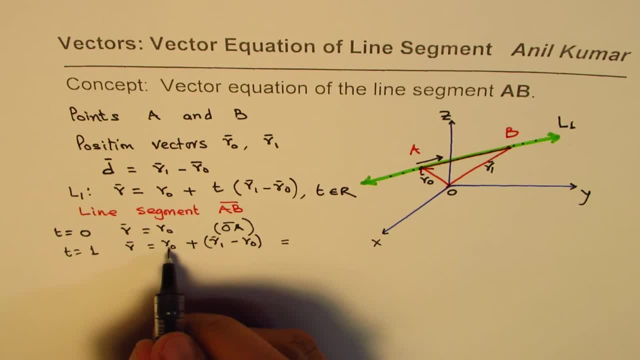 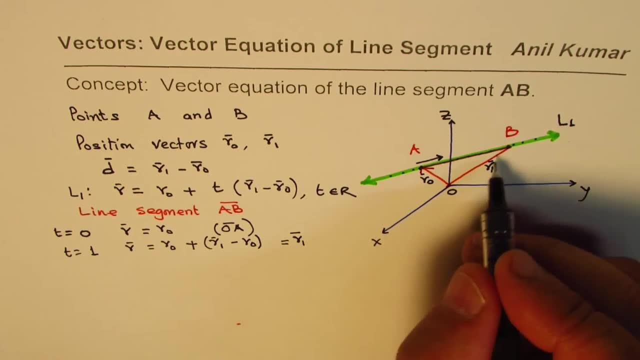 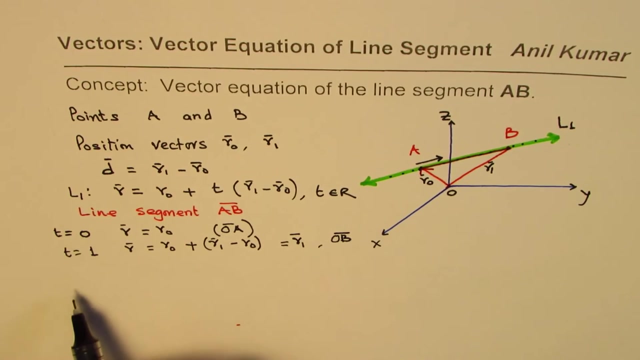 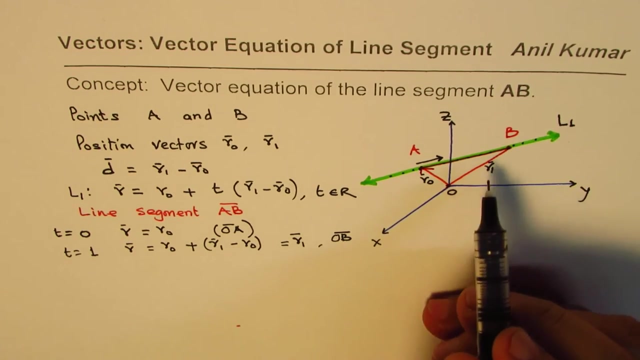 and that gives you r 0 minus r 0, 0, so we get the vector r 1, this vector which represents the position, vector ob. so what you notice here is that if t equals to 0, then it is point a, when t is 1, it is point b, and 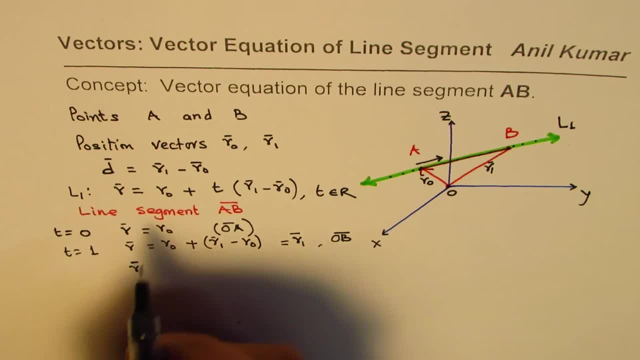 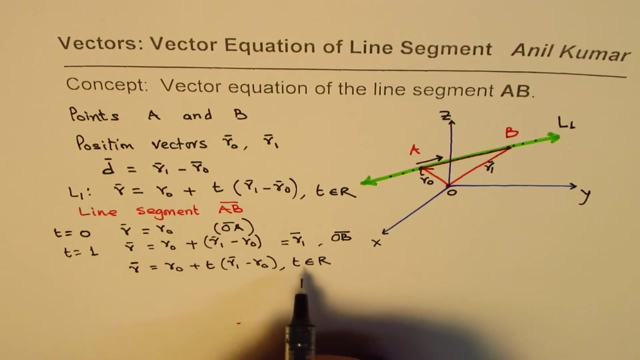 therefore, we can see that this equation, which is a general line equation- r equals to r 0 plus t times 0, r 1 minus r 0, where t belongs to real numbers, can represent the line segment, provided we give a condition that t is less than equals to 0, greater than equal to 0 and less than equal to. 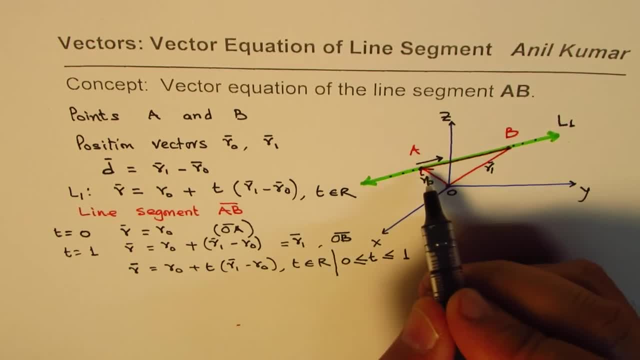 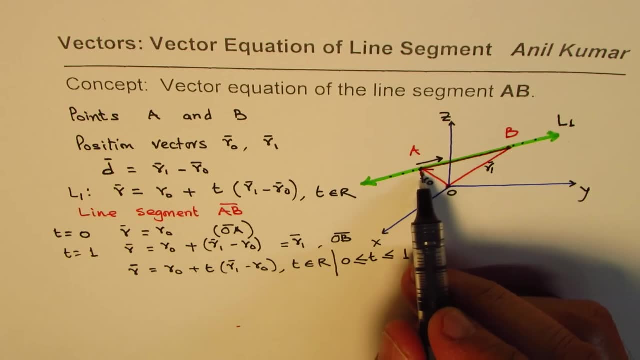 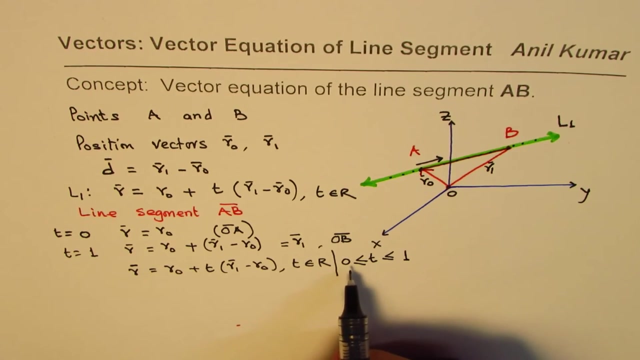 1, right? so in that case, the line segment a, b is defined. do you get the idea? so, basically, the line segment is the portion of the line where the parameter t is within 0 and 1, right? so that is what it is. sometimes we do rearrange this equation. let me do that. but this is also the right equation. 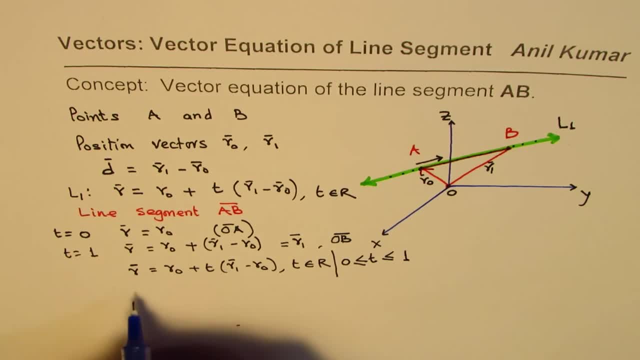 for the line segment. let me rearrange and write it. so we write this also: as r equals to r 0, we open the bracket so we get plus t r1, minus t r0. right, these are vectors. and then we can take r0, r0. 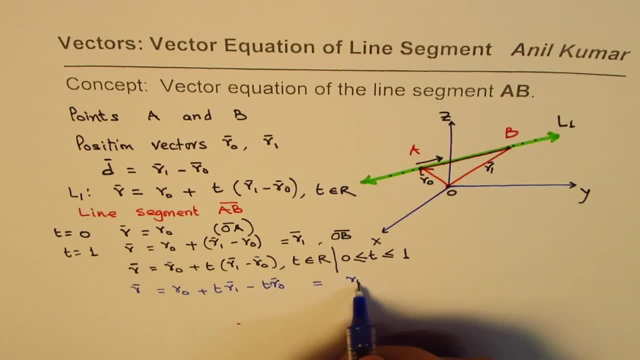 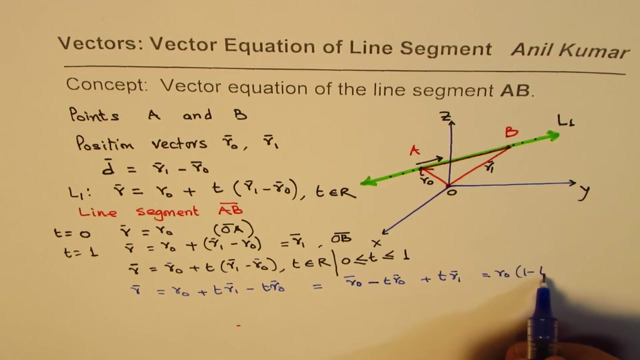 comma, so we can write this as r0 minus t r0. let me rearrange and then i'll write down: plus t r1. if i take r0 common, i get 1 minus t plus t r1, right? so this is another way of writing the.